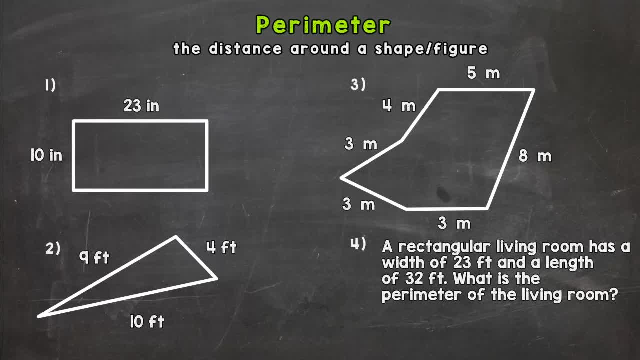 perimeter of something. all you need to do is add up all of the sides. So we have four examples here on your screen that we're going to go through in order to get this down. So let's take a look at number one. here We have a rectangle, and a rectangle has four sides, so we need to add all four sides up. 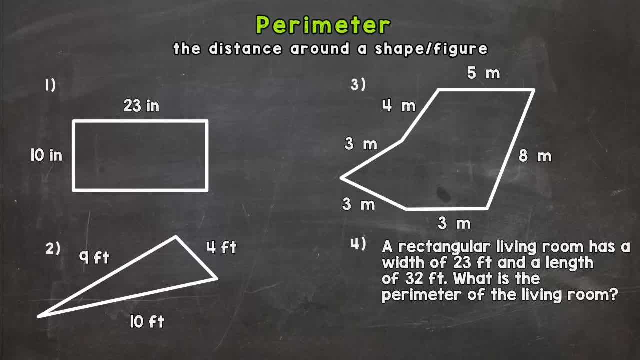 to find the perimeter. Now we have a 10 inch here and a 23 inch on the top of the rectangle. So, again, a rectangle has four sides, so let's fill in the two missing sides across from the 10 inches. This is the 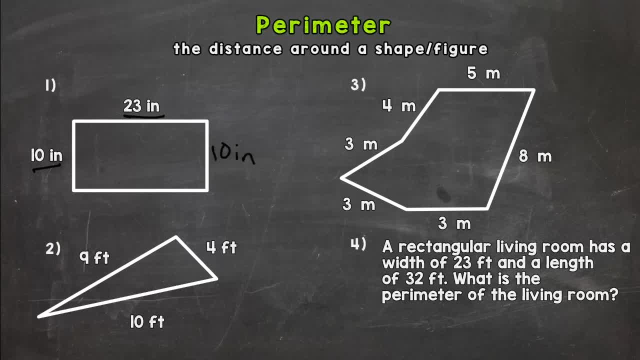 same. so we have 10 inches over here and then we need to fill in the bottom, which is 23 inches, the same as the top, So our perimeter equals the sum of all four sides. so we need to add them up So we have 23 plus 23 plus 10 plus 10.. So we need to write perimeter equals and then let's find the. 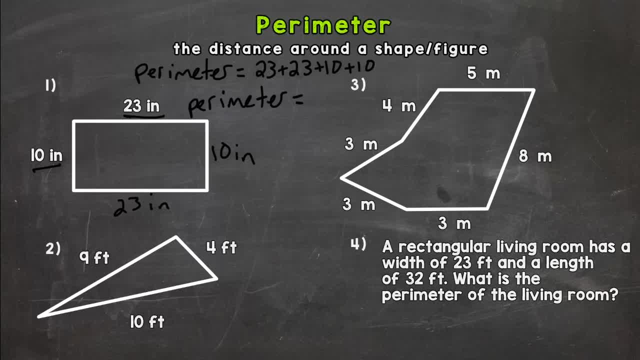 sum. So 23 plus 23 is 46, plus 10 is 56, plus another 10 is 66.. Now another important thing: when it comes to perimeter in your final answer, we need a unit of measure. So look back in the original problem. 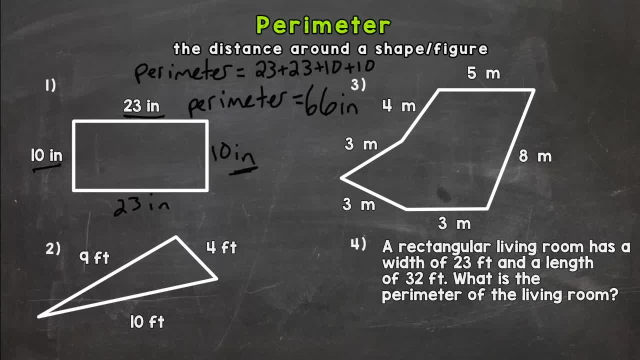 and we're working with inches, So we need to label our answer: perimeter equals 66 inches. Again, perimeter equals 66 inches, So we need to label our answer: perimeter equals 66 inches, So we need to label our answer. perimeter equals 66 inches, So we need to label our answer: perimeter equals 66 inches. 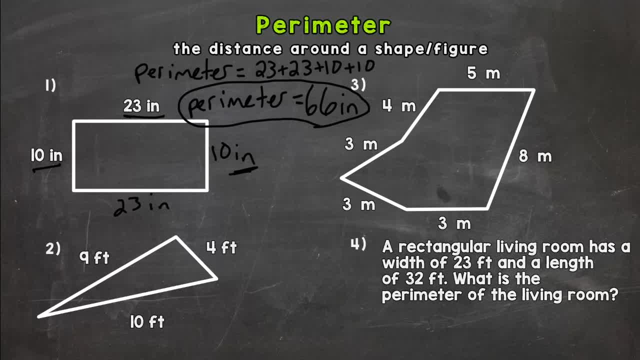 Last answeriren, you need to remember to have all of the sides included. so I'm going to have one perimeter the distance around a shape or figure. Sir, we have 24 sides and we have two sides for Het, We have 24 sides for here. So perimeter equals 66 inches plus first. 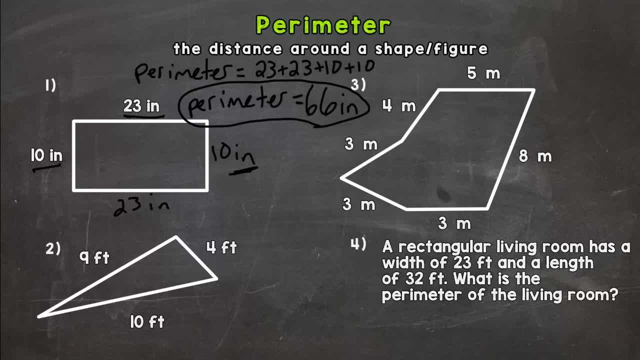 perimeter equals 66 inches plus 10 plus 2 inches. This is time And you need to remember to make sure you include all of the sides. So for number one, we had four sides. Let's take a look at number two. We have 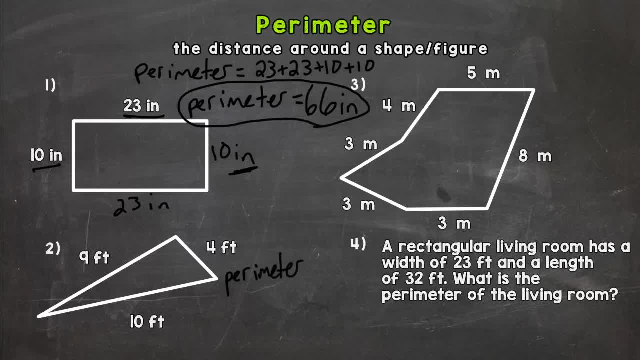 a triangle. The problem that I'm dealing with here is that when we look at every side of this perimeter and we paint, the image is that all of the sides, we're nothing but in the top. So perimeter is going to equal the sum of all the sides and we have one, two, one, two, three sides. 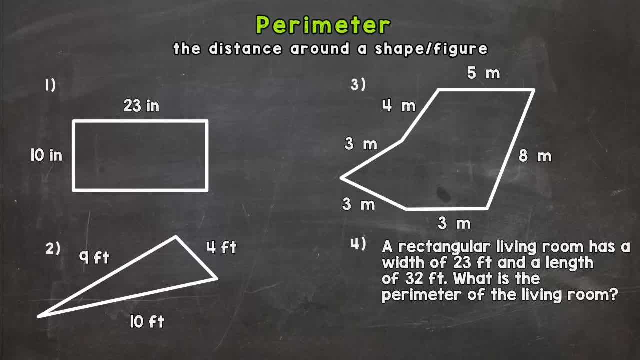 to find the perimeter. Now we have a 10 inch here and a 23 inch on the top of the rectangle. So, again, a rectangle has four sides, so let's fill in the two missing sides across from the 10 inches. This is the 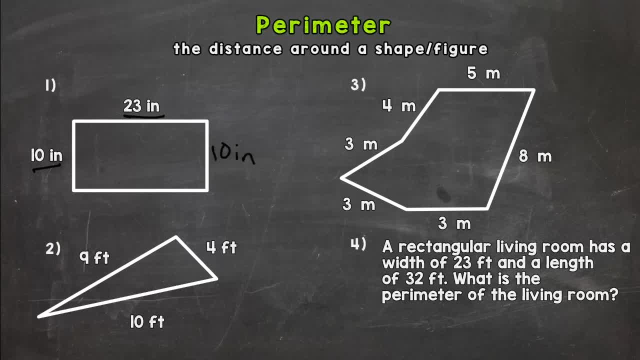 same. so we have 10 inches over here and then we need to fill in the bottom, which is 23 inches, the same as the top, So our perimeter equals the sum of all four sides. so we need to add them up So we have 23 plus 23 plus 10 plus 10.. So we need to write perimeter equals and then let's find the. 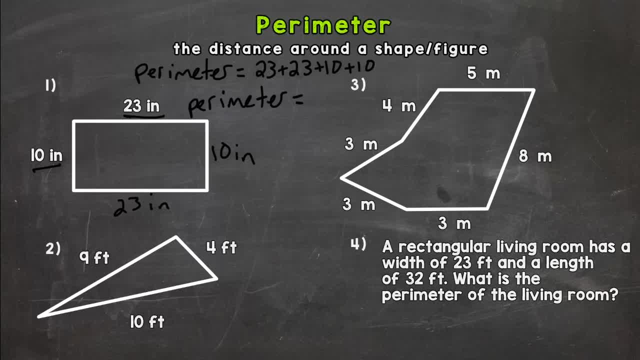 sum. So 23 plus 23 is 46, plus 10 is 56, plus another 10 is 66.. Now another important thing: when it comes to perimeter in your final answer, we need a unit of measure. So look back in the original problem. 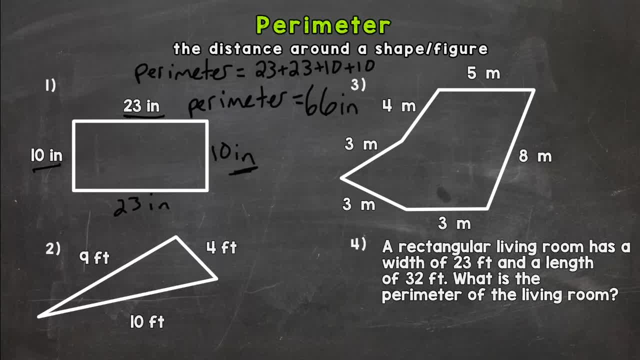 and we're working with inches, So we need to label our answer: perimeter equals 66 inches. Again, perimeter equals 66 inches, So we need to label our answer: perimeter equals 66 inches, So we need to label our answer. perimeter equals 66 inches, So we need to label our answer: perimeter equals 66 inches. Again. 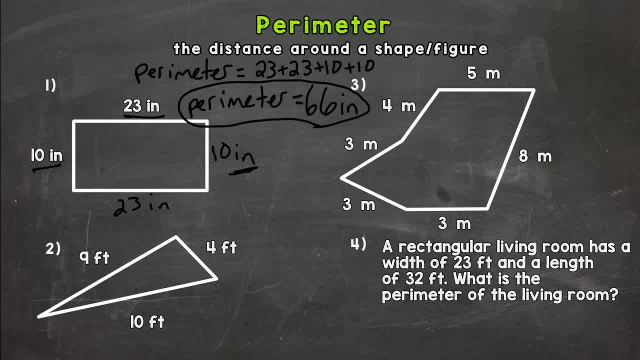 primera, the distance around a shape of shape or figure, and you need to remember to make sure you include all of the sides. So for number one, we have four sides. Let's take a look at number two. You have a triangle, So perimeter is going to equal the 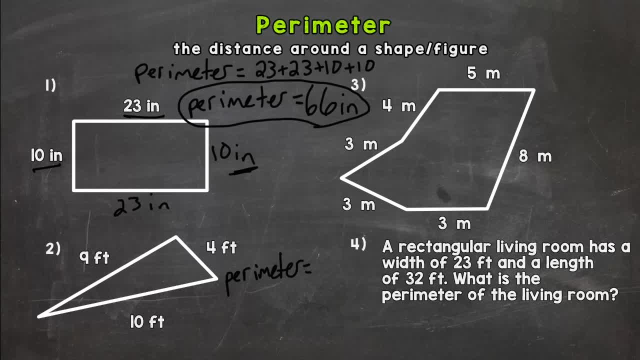 sum of all the sides, and we have one to 123 sides. So we need a nine plus a, four plus a, And 18 and 19.. a four plus a ten, a four plus a ten- 10. so let's add those up: 9 plus 4 is 13 plus 10. we get 23 and we need a unit of. 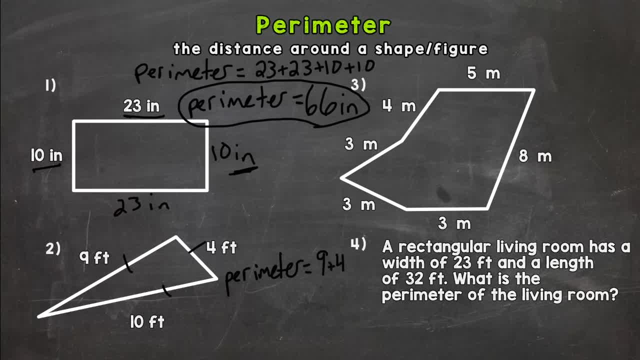 So we need a nine plus a 4, plus a 10.. So let's add those up: 9 plus 4 is 13, plus 10, we get 23.. And we need a unit of measure which is feet. 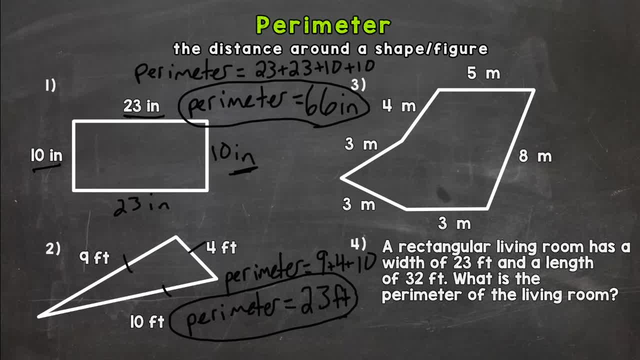 So the perimeter or distance around that triangle is 23 feet. Let's look at number 3 here. Now this one. you need to make sure to include all the sides, make sure you don't forget any of the sides right, And then don't repeat anything. 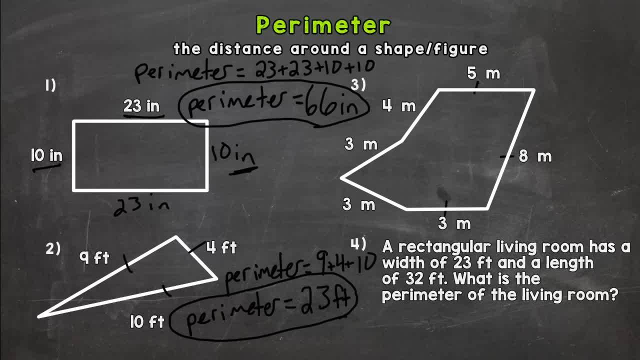 So let's see how many sides we have: 1,, 2,, 3,, 4,, 5,, 6 sides. So that means we need 6 numbers added up. So let's start up top. We have a 5.. 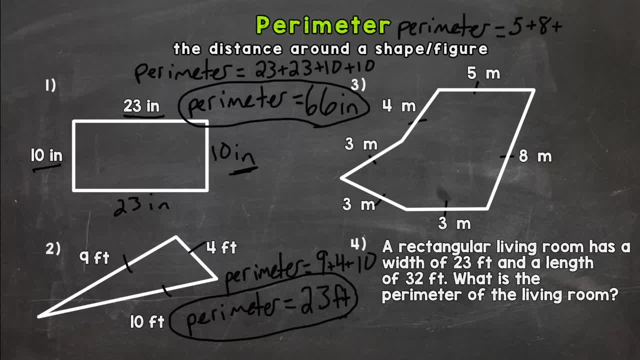 Plus 8,, plus the bottom 3,, plus another 3,, plus another 3, and then a 4.. Let's see if we have all 6.. 1,, 2,, 3,, 4,, 5,, 6.. 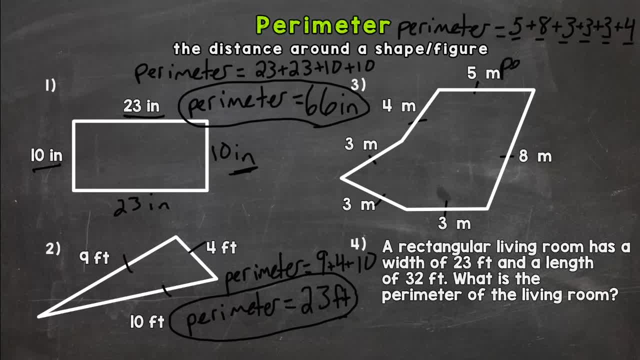 It never hurts to double check. Alright, let's find the sum, and that will be our distance around that six-sided figure. And a six-sided figure is called a hexagon. So 5 plus 8 is 13,, plus 3 is 16, plus another 3 is 19,. 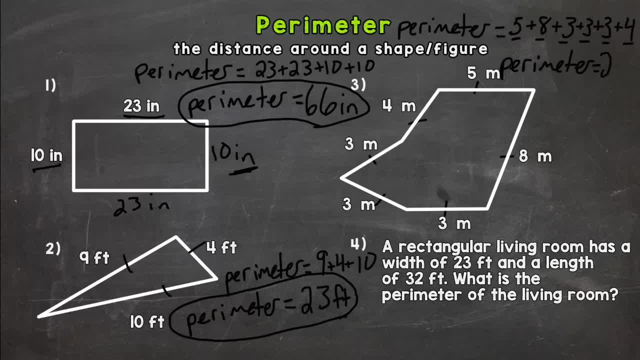 plus 3 is 22, plus a 4. We get a perimeter of 26,, and this M stands for meters, So a perimeter of 26 meters. Alright, number 4, we have a little word problem here- A rectangular. 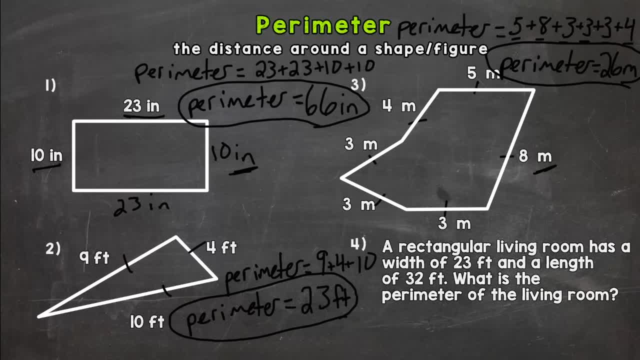 living room has a width of 20 meters 23 feet and a length of 32 feet. What is the perimeter of the living room? So I would suggest, whenever you have a situation given, draw a picture in order to help us start this problem. 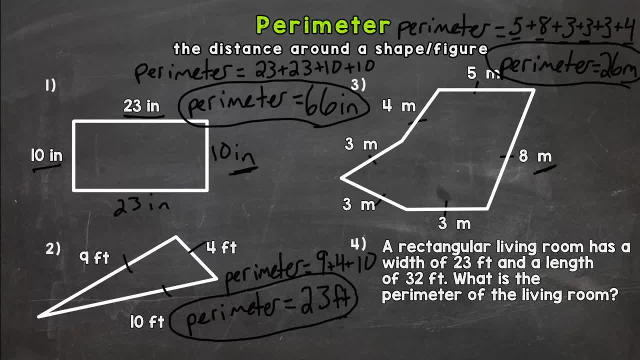 and make sure we have the correct answer and everything's set up correctly. So it says rectangular living room. So I'm just going to draw a rectangle here- Not perfect straight lines, but it will work. So it has a width of 23 feet and a length of 32 feet. 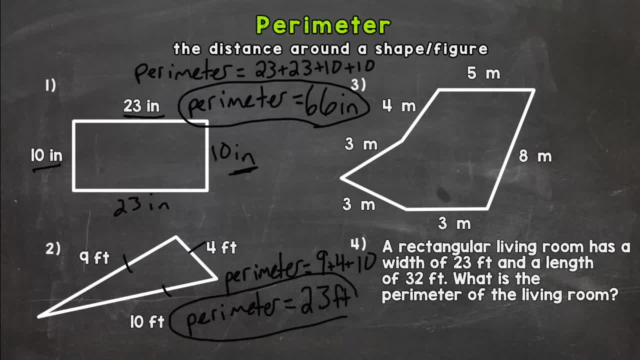 measure, which is feet. so the perimeter or distance around that triangle is 23 feet. let's look at number three here now this one. you need to make sure to include all the sides, make sure you don't forget any of the sides right and then don't repeat anything. so let's see how many sides we have: 1, 2, 3, 4, 5, 6 sides. 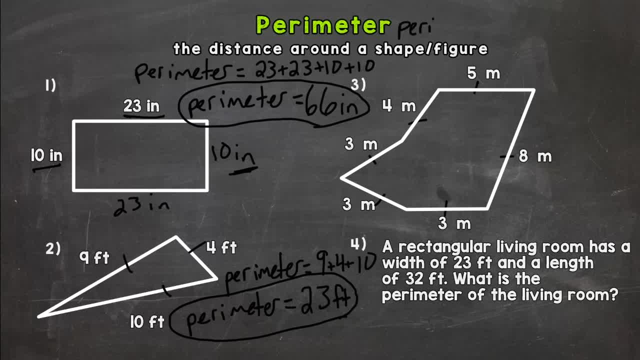 so that means we need 6 numbers. add it up. so let's start up top. we have a 5 plus 8, plus the bottom 3 plus another screen, three plus another three and then a four. Let's see if we have all six, One, two. 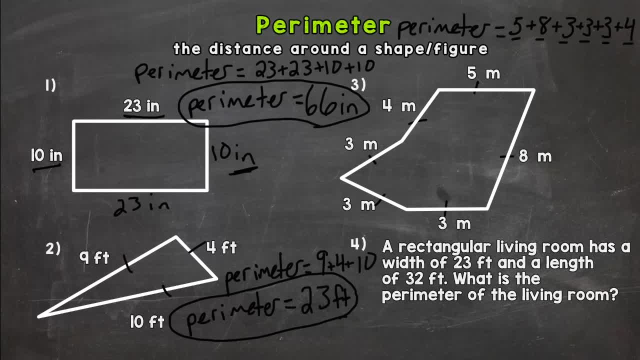 three, four, five, six. It never hurts to double check. Alright, let's find the sum and that will be our distance around that six-sided figure. And a six-sided figure is called a hexagon. So five plus eight is thirteen plus three is sixteen. 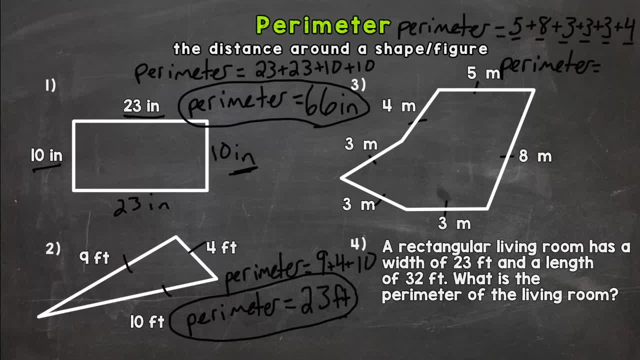 plus another three is nineteen, plus three is twenty-two plus a four, We get a perimeter of twenty-six, and this M stands for meters, So a perimeter of 26 meters. Alright, number four- we have a little word problem here: A rectangular. 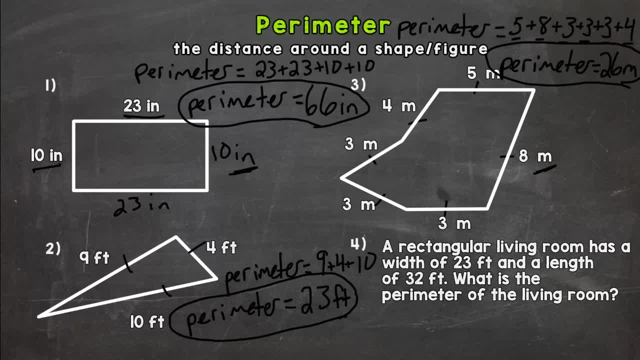 triangle. The living room has a width of 23 feet and a length of 32 feet. What is the perimeter of the living room? So I would suggest, whenever you have a situation given, draw a picture in order to help us start this problem and make sure we have. 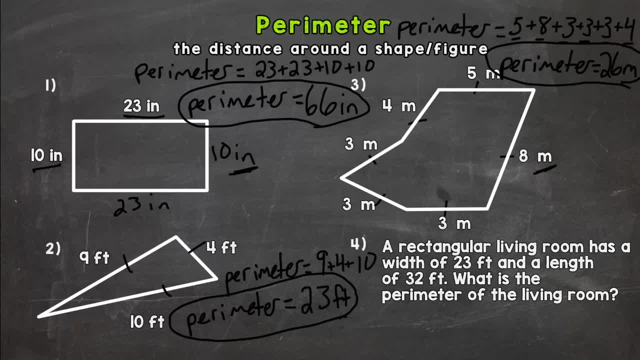 the correct answer and everything's set up correctly. So it says rectangular living room. So I'm just going to draw a rectangle here- Not perfect straight lines, but it will work. So it has a width of 23 feet and a length of 32 feet. Now, if you have the